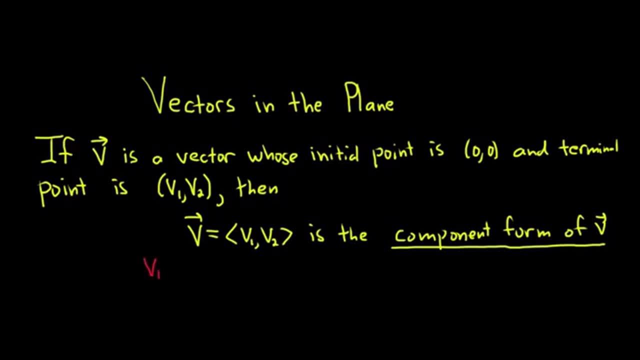 And these guys here, so v1 and v2, these guys here. these are called the components, components. You can think of the first one as x and the second one as y. We're just being a little bit more general here when we call them v1 and v2.. 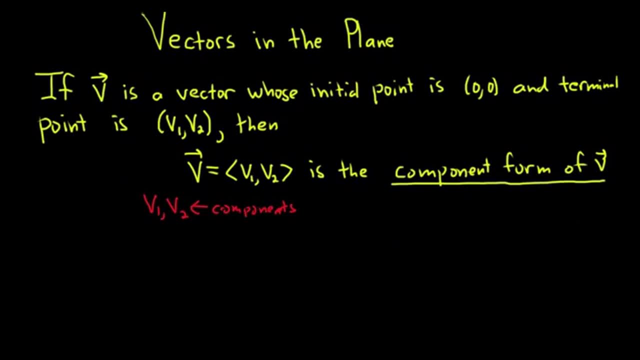 So let me give you a picture so you see what's going on. So here's the pic. So here we have the y axis and here we have the x axis. So x, y and y. So here we have the y axis and here we have the x axis. 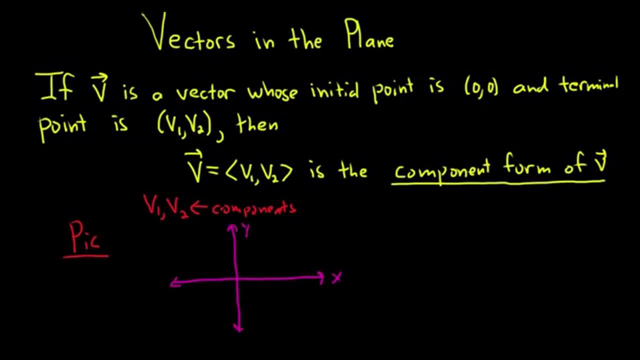 So here we have the y axis, and here we have the x axis, And then maybe this is the initial point, and then this is what's called the terminal point. So this point here would be v1,, comma v2.. And so our vector would look something like this: okay, 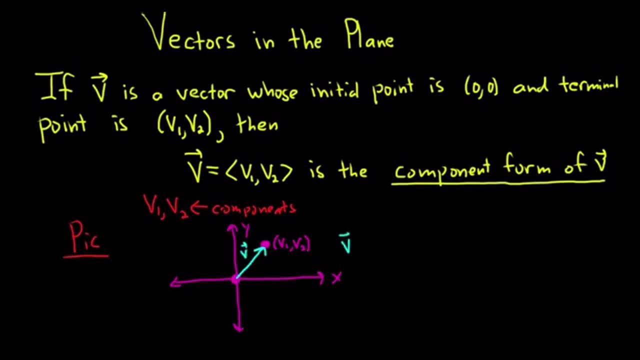 And that would be our vector v. So you could say v in this case is the vector whose first component is v1 and second component is v2.. Since the initial point here is at the origin, I did that on purpose. then we say that our vector is: 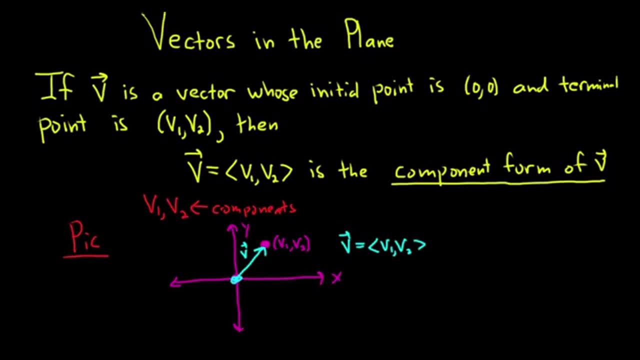 in standard position. So this is a vector in standard position because the initial point is the origin. okay, So let me go ahead and write that down. So, since the initial point is the origin, we say the vector is in standard position. We say the vector is in what's called standard position. 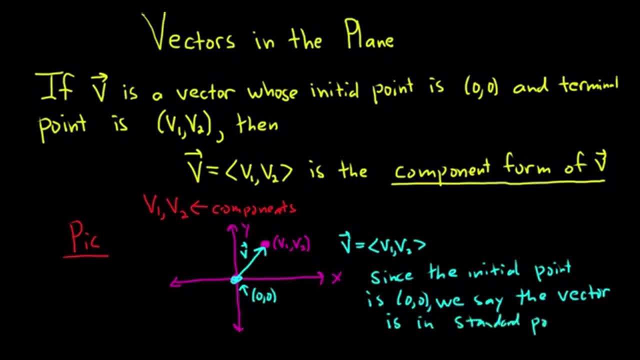 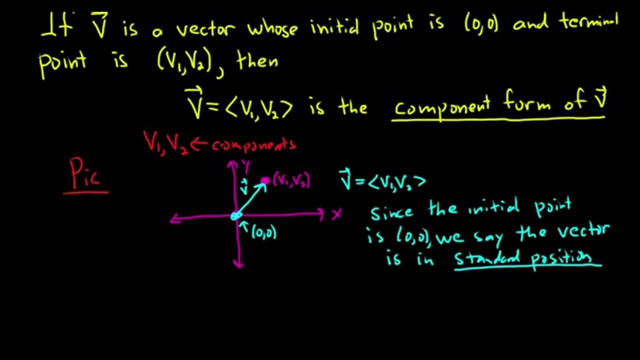 So standard, standard position, Okay, lots of terminology, but it's good stuff, It really really is. It really really is. Just a quick aside or just another remark. actually The vector with initial point zero, zero and terminal point zero. 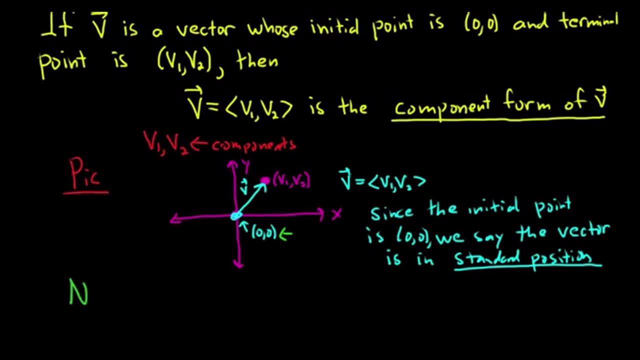 Point zero, zero is called the zero vector. So note the vector with initial point and terminal point zero, zero. So the initial point is the same as the terminal point and they're both zero, zero. It's called the zero vector. It's a very important vector in calculus three. 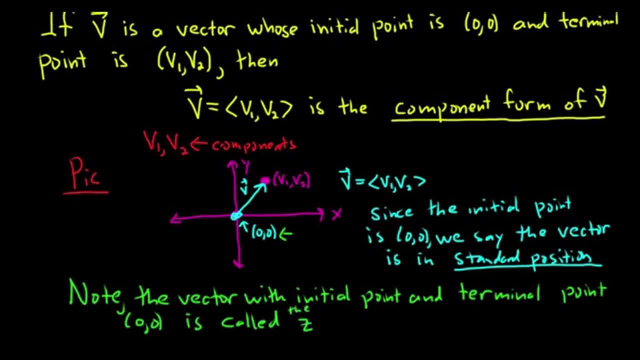 and in mathematics It's called the zero. it's called the zero vector. Okay, we're going to use it a lot And the notation for the zero vector is a zero. right, It's a zero, but since it's a vector, 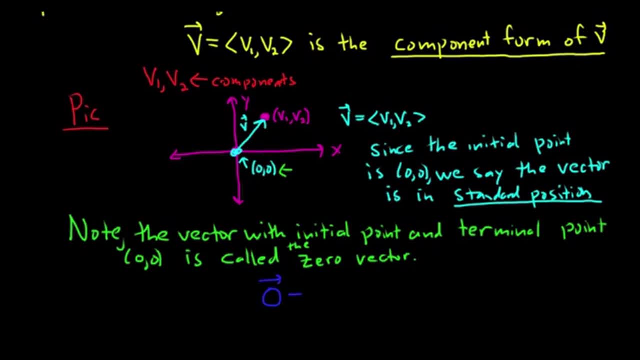 we put a line with an arrow above it And the first component of the zero vector is zero and the second component of the zero vector is also zero. So very, very special vector In the world of vectors. Let's look at another picture that's going to prove. 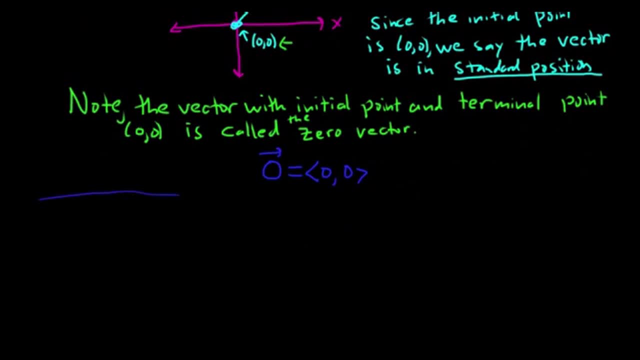 to be useful, especially later on if you're trying to understand the derivations of some of the formulas in calculus three. So a worthy picture. So consider the following picture. Okay, say we have a vector here, Starts here and ends here. 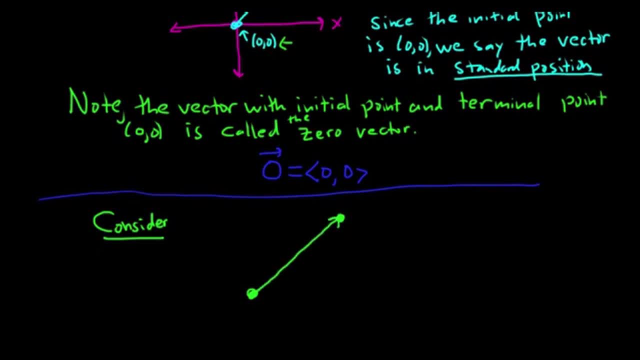 So I'll connect the dots and draw the vector And say the initial point here. in this case we'll call it P And I'll say the components of P are P1, P2.. So it's not a vector, sorry, I said components. 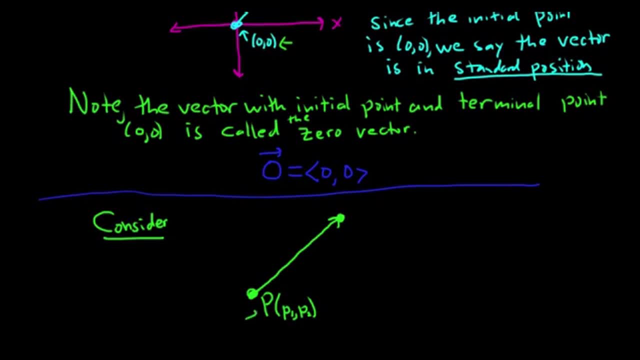 The coordinates of P. So the X coordinate of the point P is P1, the Y coordinate is P2.. And here we have another point Q. This is our terminal point, And the coordinates of this point are Q1, Q2.. 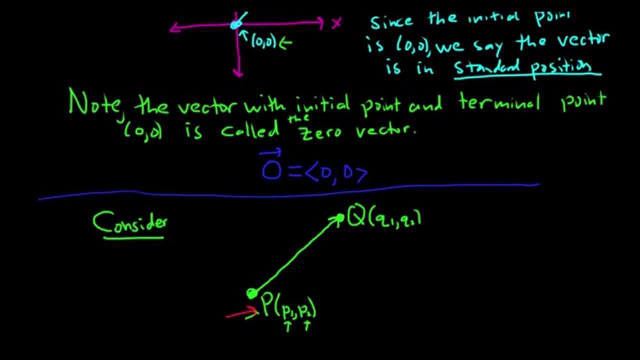 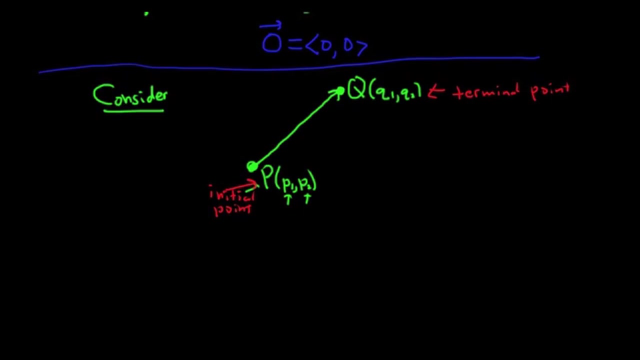 So this is the initial point here. So P is the initial point And Q is the terminal point. terminal point: Okay. so we have a vector with initial point P and terminal point Q. okay, And the idea is this: To find our vector V. here's the thinking you want. 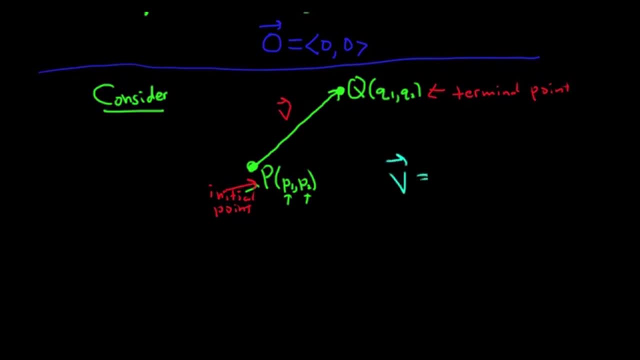 to go through in your head. V is always going to be- I'm going to put this in quotes- it's always terminal. terminal minus initial. You can always do that every single time, all day long, right? Terminal minus initial. terminal minus initial. 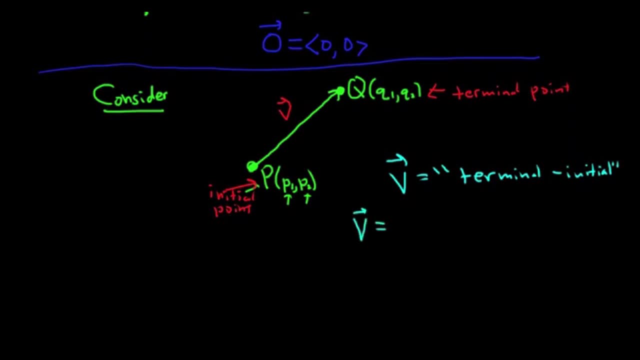 So, more formally, to find the vector V, what you do is you take the terminal, so Q1 minus P1.. So you subtract the first components, okay, So Q1 minus P1.. And then you subtract the second components, So Q2 minus P2.. 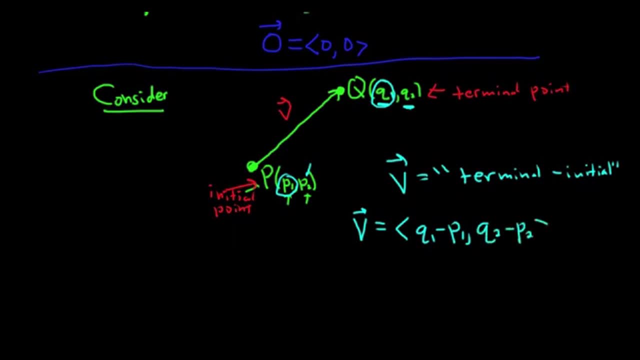 You can always do that. So Q2 minus P2.. Okay, And that gives you your vector right, And this is V1 comma V2.. So we're saying that this here is V1 and this here is V2.. This is super useful, okay. 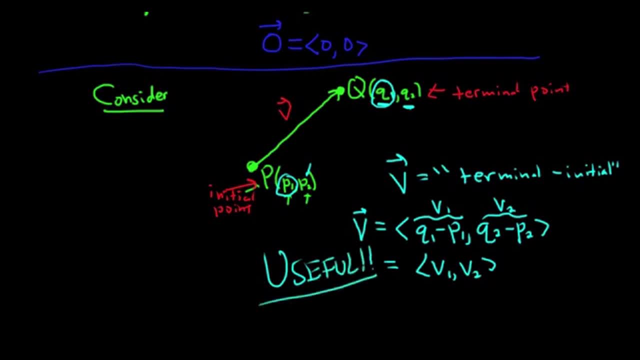 Extremely. you kind of emphasize how useful this thinking is. So if you ever have an initial point and a terminal point, it's always terminal minus initial. to get the vector: to get the vector. All right, there's a couple of formulas. 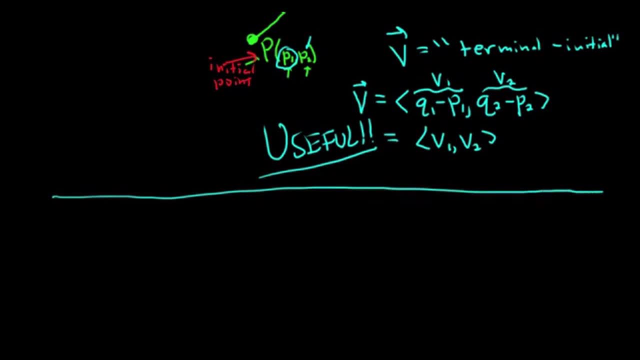 Sometimes we're interested in finding the initial point. Sometimes we're interested in finding what's called the length of the vector. So the length, it's also called the norm. okay, It's also called the magnitude. So lots of names for the same thing. 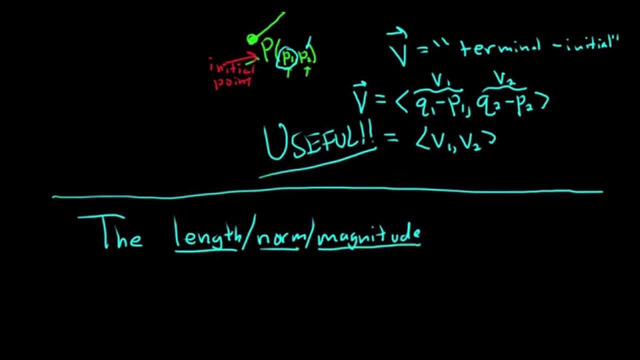 So the length, norm, length, norm slash, magnitude of a vector, let's call our vector V, And component form it would be, I suppose, V1 comma, V2.. And what you do is you write these two double bars and you put the V here, double bars. 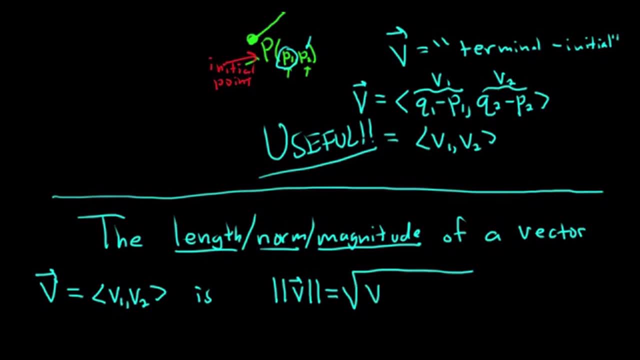 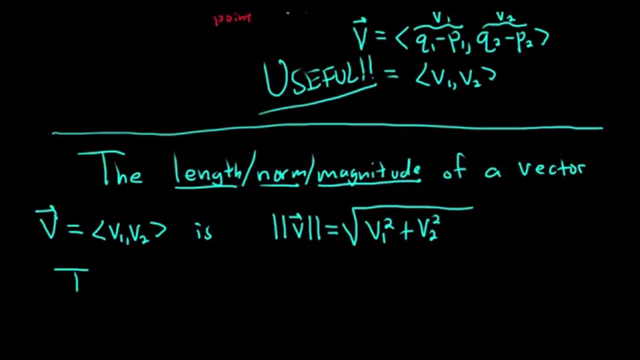 And it's the square root of the components squared, So V1 squared plus V2 squared. okay, That's the length norm or the magnitude of a vector, If the magnitude is 1 or if the norm is 1 or if the length is 1,. 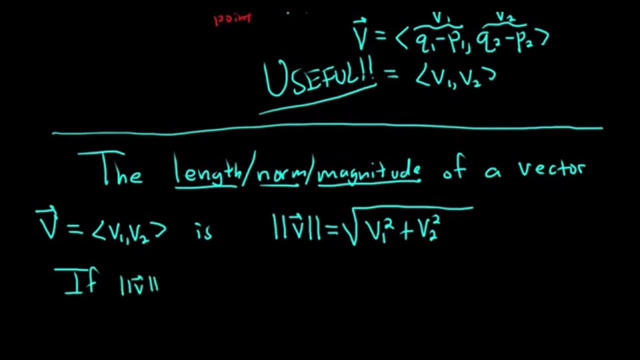 depending what you want to call it. So if you have a vector with magnitude 1, whenever that happens, okay, whenever that happens you have- then V is a unit vector. Then V is a unit vector Really important. And the reason it's important is because unit vectors are nice. 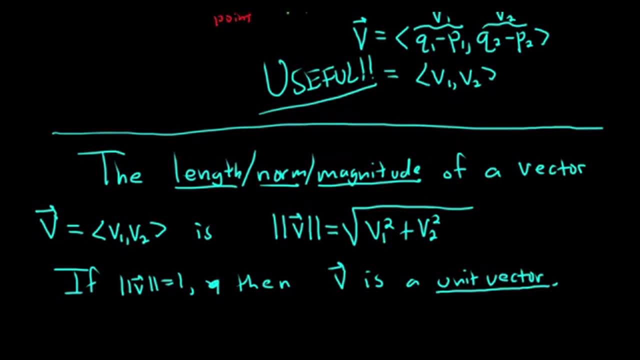 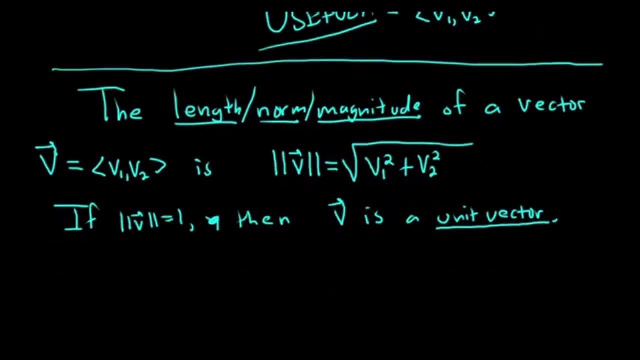 right Whenever you have 1 as the magnitude. it simplifies the formulas right, Simplifies them tremendously, tremendously. So let's just do a really simple example of computing the magnitude, Just a simple, simple problem. Say we have the vector of V equals 1 comma 2.. 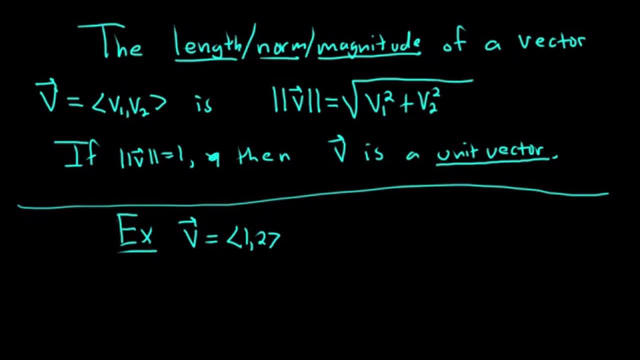 So in this case, if we wanted to find the magnitude, what we would do is we would just square the components and take the square root. So the magnitude of V, in this case it's the square root of 1 squared plus 2 squared. 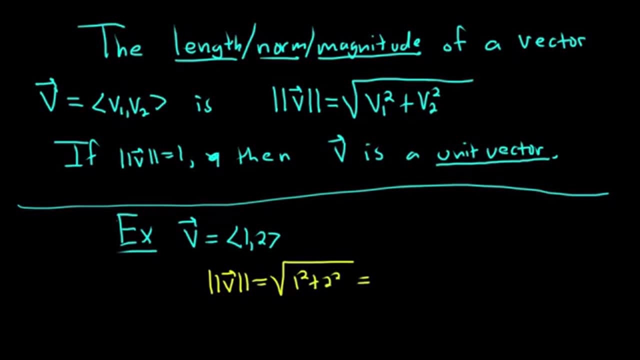 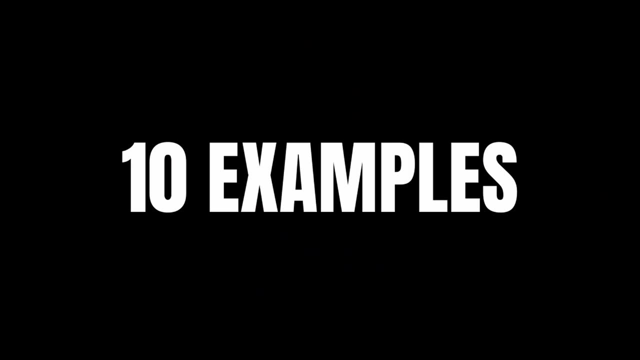 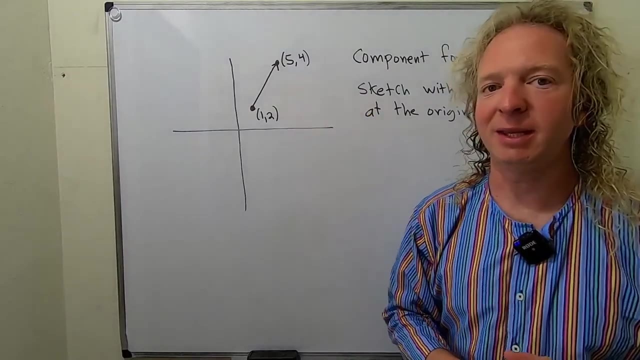 Okay, So you just do 1 plus 4, and so you get the square root of 5, and that would be the magnitude. In this video. we have a vector written in the plane and we have to find the component form of this vector. 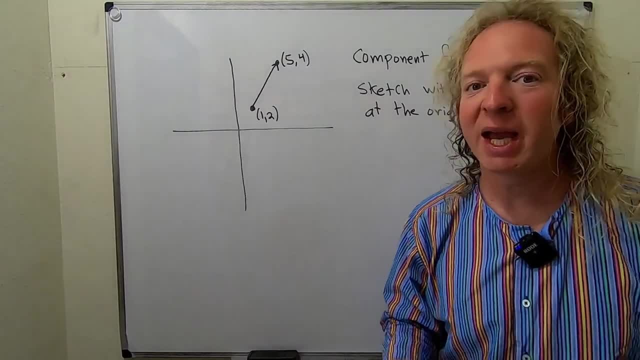 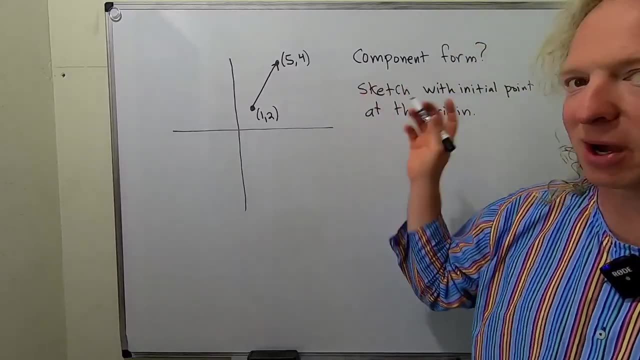 and we also have to sketch the vector with its initial point at the origin. So this problem may be simple, but it does illustrate a a super, super important concept. So let's go ahead and write the component form down first. So the component form of our vector, which I'll call V. 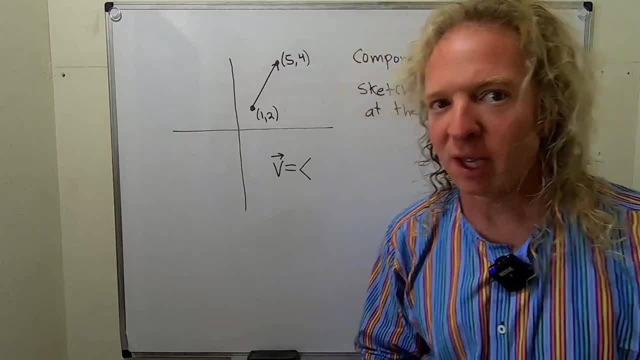 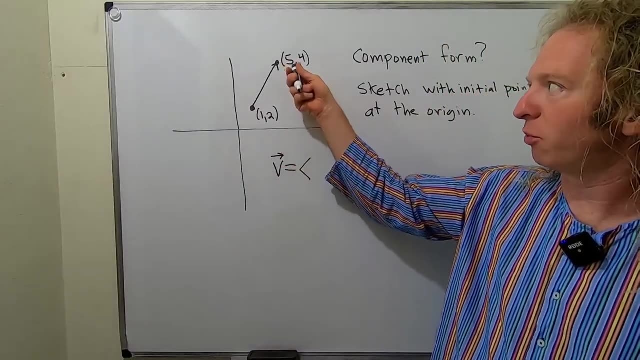 is equal to angle bracket and there's a formula: It's always terminal minus initial, So terminal minus initial. So in this case you look at the terminal point, That's this one. That's where it ends and this is the initial point. 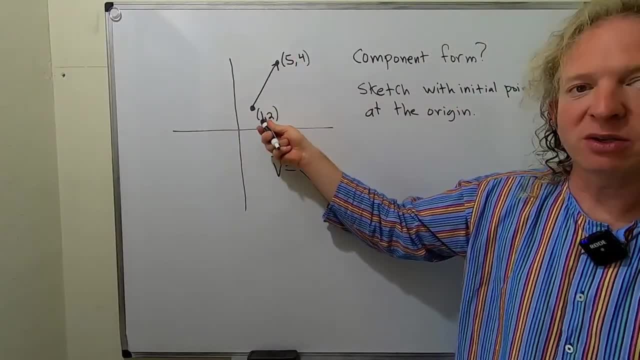 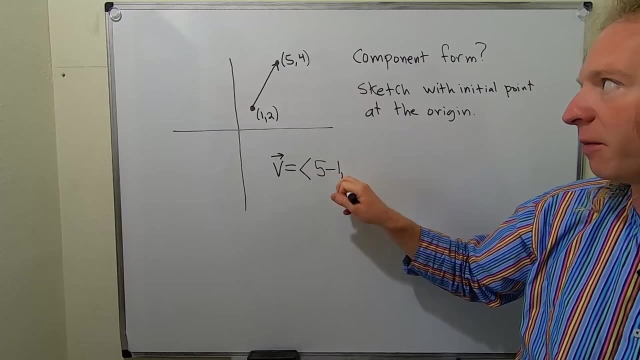 This is where it begins. So it's this one minus this one. So you subtract the components, So you do 5 minus 1.. So I'll write it 5 minus 1, and then 4 minus 2,, 4 minus 2.. 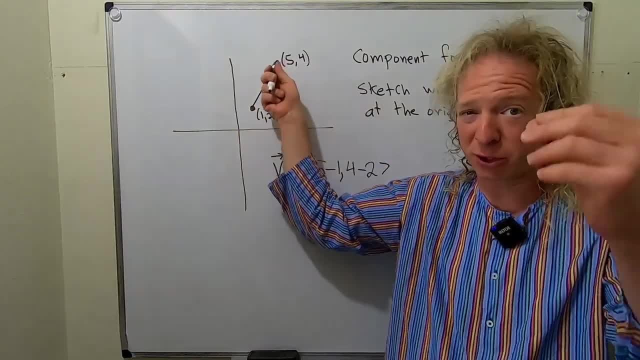 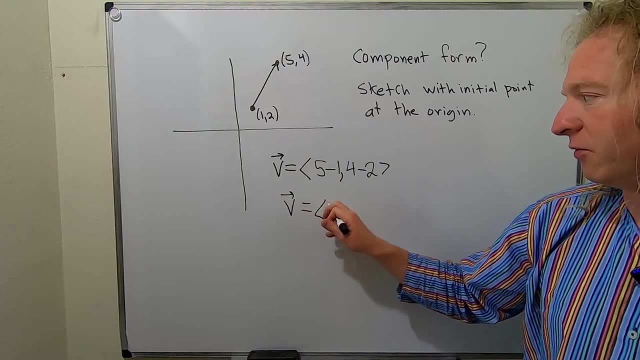 So you subtract the x components and you subtract the y components, or the first components and the second components, Terminal minus initial. So we end up with V equals. this would be 4 comma 2.. The question doesn't ask, but if we wanted to write it, 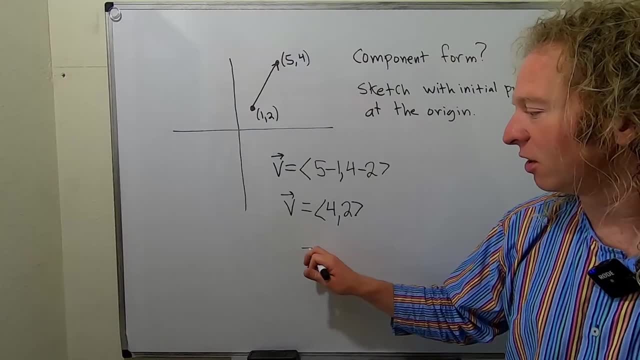 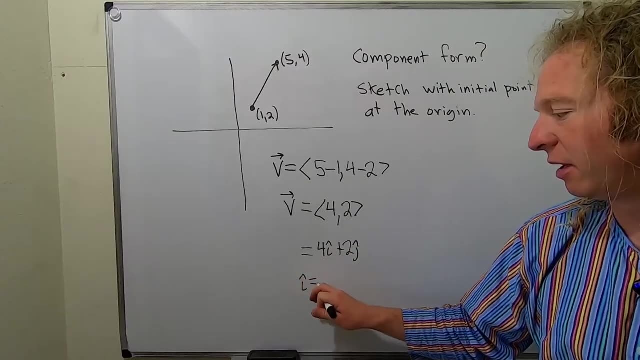 as a linear combination of i and j. so if we know what that is, you could write it like this: 4 i hat plus 2 j hat. And as a refresher, i hat is this vector: here It's called a unit vector because it has length 1.. 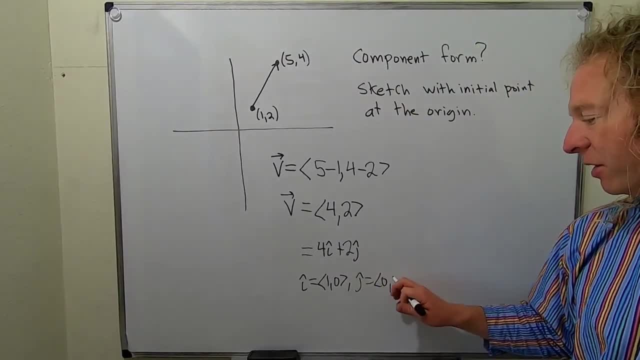 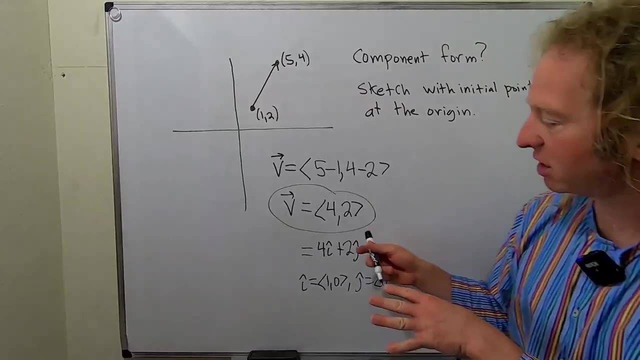 And then j hat would be this unit vector here. These are called the standard unit vectors. Anyways, this is not what we needed in this problem. Okay, so now we have to sketch this with the initial point at the origin. It's a pretty easy sketch. 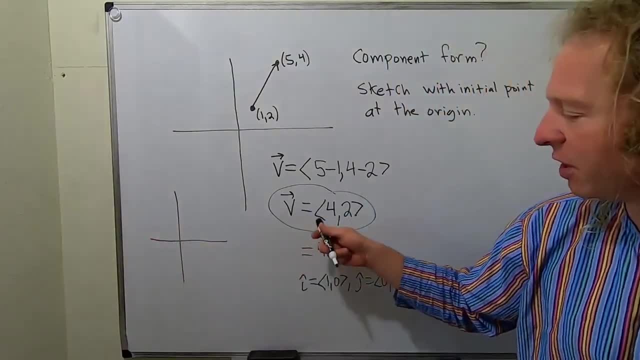 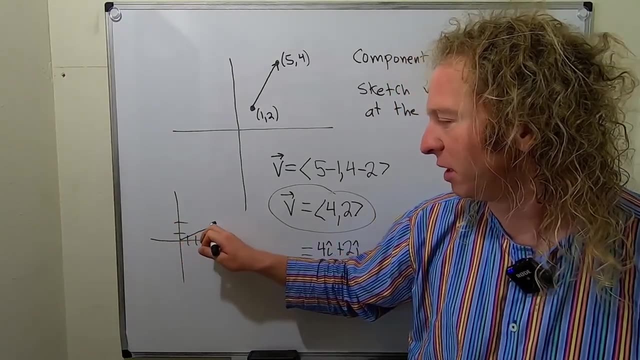 I'll do it over here. So there's the y axis, There's the x axis, So 4, 2.. So you just go right 4 and up 2, and you put a dot there And that would be your vector there. 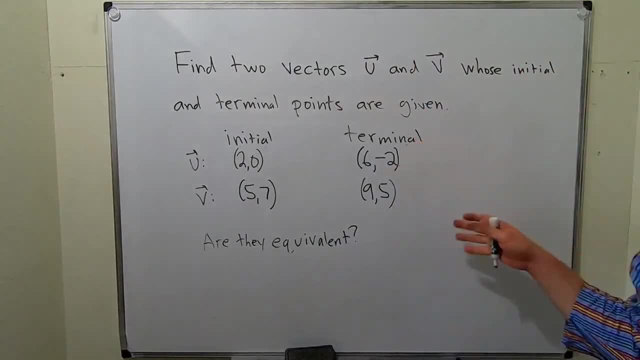 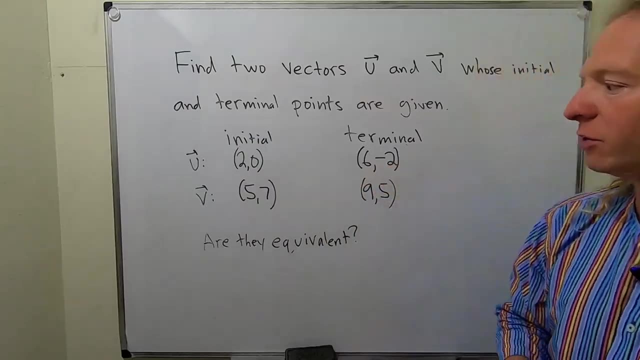 I hope this video has been helpful. Find two vectors, u and v, whose initial and terminal points are given. So we have a vector u whose initial point is 2, 0, and terminal point is 6, negative 2.. 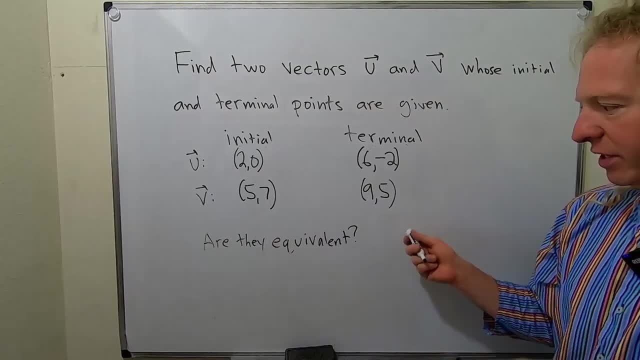 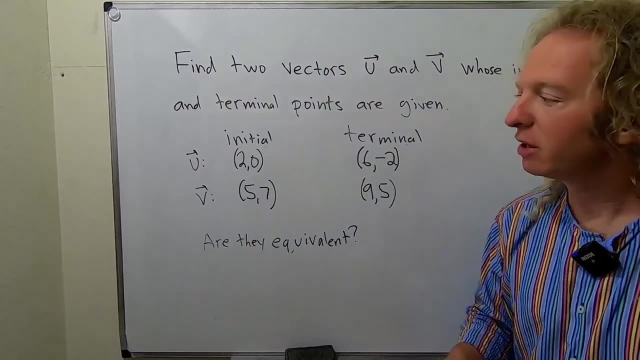 And a vector v whose initial point is 5, 7, and its terminal point is 9, 5.. And there's a follow-up question that says: are the vectors equivalent? Two vectors are equivalent if they have the same magnitude and direction. 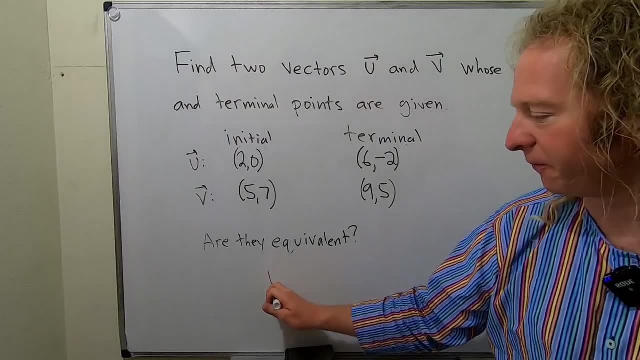 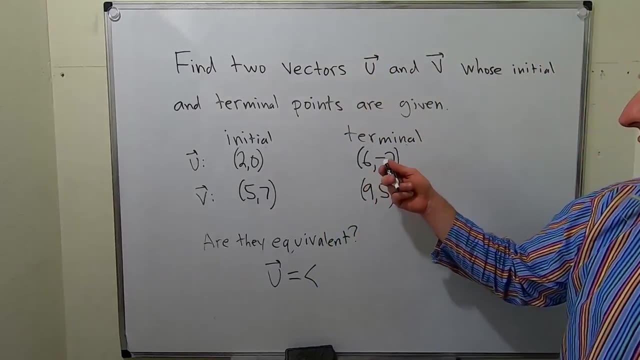 So let's go ahead and find u and v. So to do that, all we have to do is subtract. The formula is always going to be terminal minus initial. So we take this point and subtract it from this point, And you just subtract the coordinates. 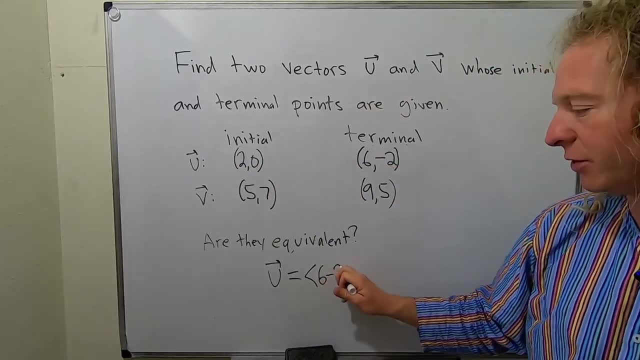 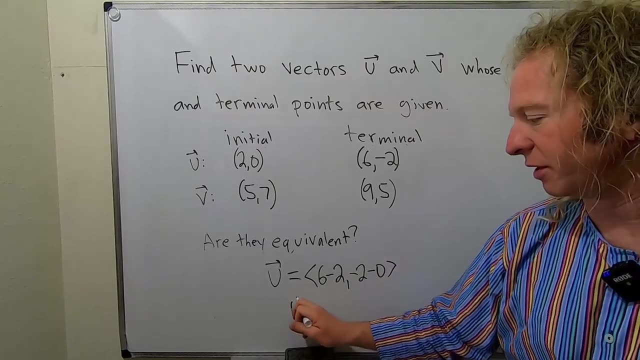 So you do 6 minus 2.. So 6 minus 2.. And then you do negative 2 minus 0. So negative 2 minus 0. So this is going to give us. let's see, 6 minus 2 is 4.. 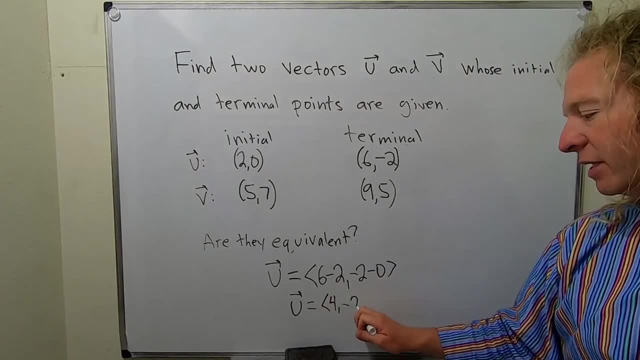 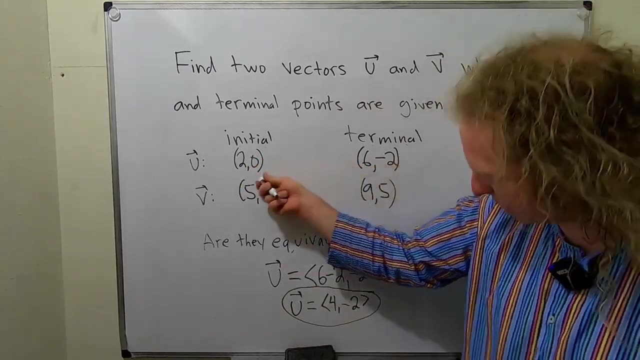 And negative. 2 minus 0 is negative 2.. So that would be our vector u. So let's just check that 6 minus 2 is 4.. Negative 2 minus 0 is negative 2.. Good stuff, Let's do v up here. 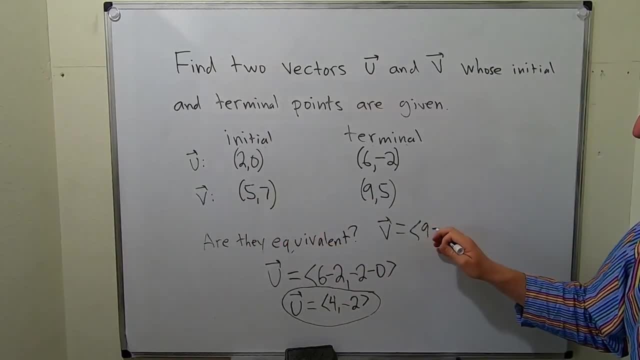 So it'll be 9 minus 5, which is 4.. I'll go ahead and I'll show the work: 9 minus 5.. And then 5 minus 7.. So 5 minus 7.. This will be: 9 minus 5 is 4.. 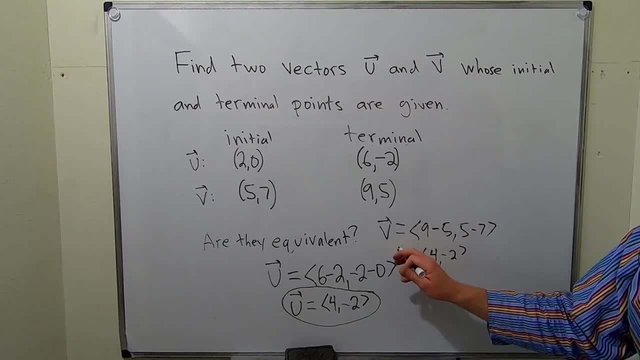 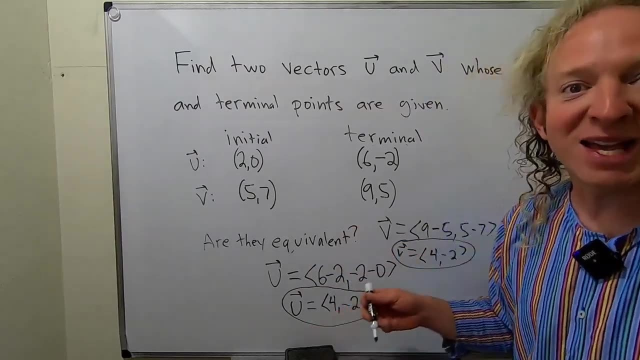 5 minus 7 is negative 2.. So this is our vector v. So we have our vector v. These are exactly the same vector. It's the same components and everything. So yes, they are equivalent. So two vectors are equivalent if they have the same magnitude. 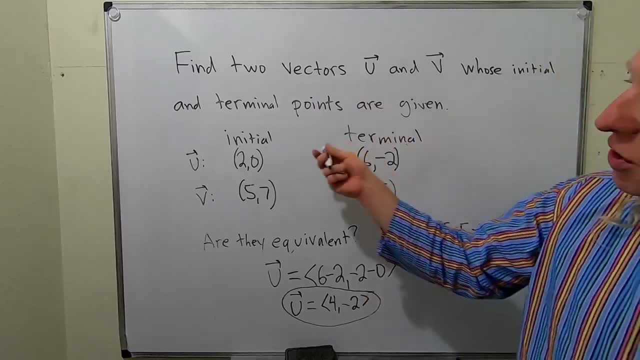 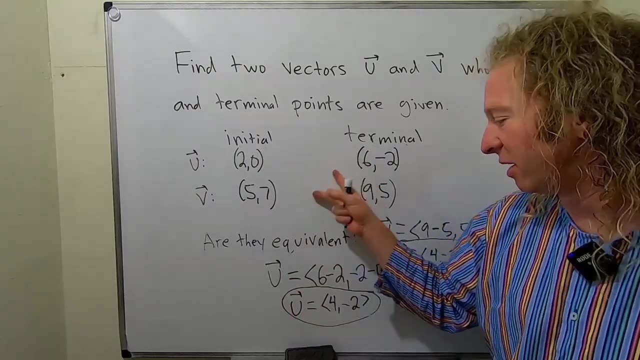 and directions. You might say: well, they're the same, So obviously they're equivalent. The question is really asking about these, These vectors here u and v are the same as these. It's the same vector, It's just in a different place. 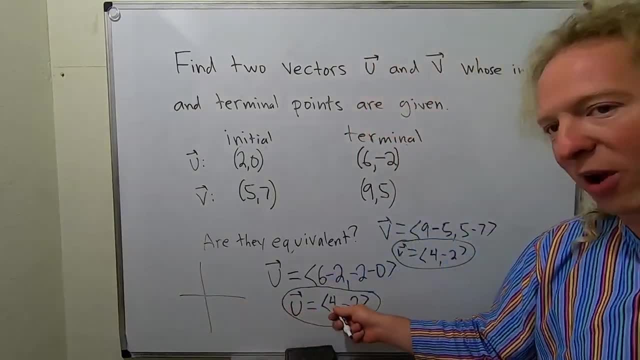 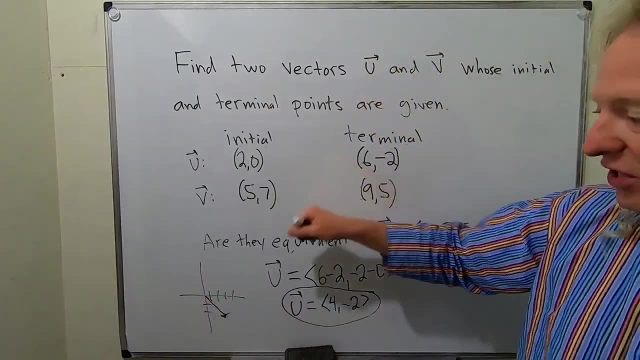 So this vector, here you go right 4 and down, 2.. So 1, 2,, 3, 4.. 1, 2.. Looks like this, Same as this one. So what are these? They're the same thing. 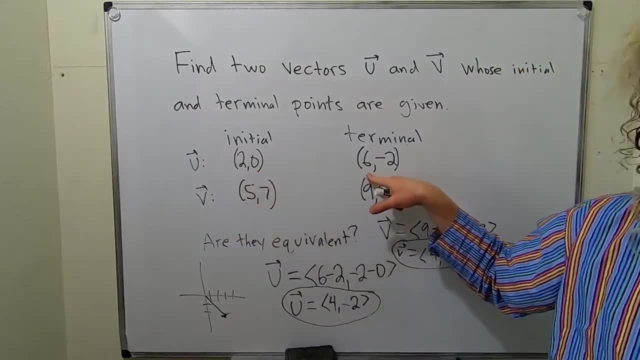 It's just they're somewhere else. The initial point here is 2, 0.. And the terminal point here is 6, negative 2.. So it's just like you've taken this vector and you've put it in a different position on the plane. 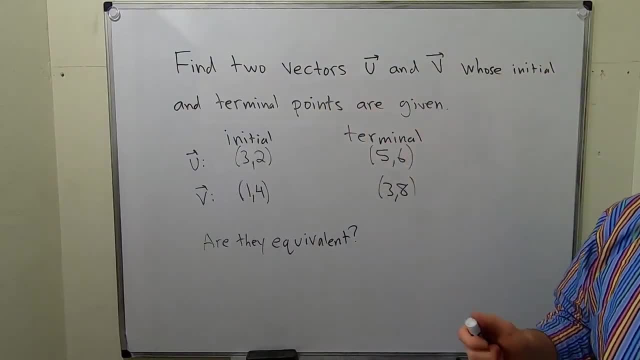 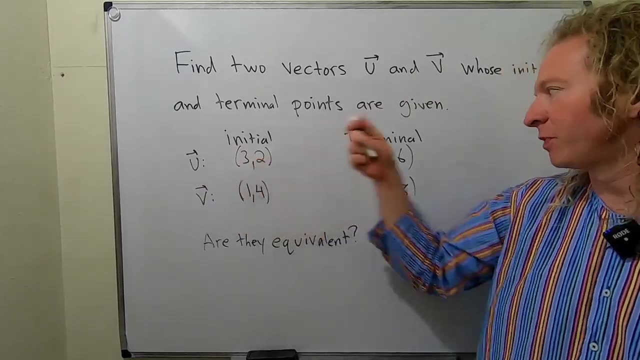 So it's the same thing. I hope this video has been helpful. Find two vectors, u and v, whose initial and terminal points are given. So we have the vector u with initial point 3, 2 and terminal point 5, 6.. 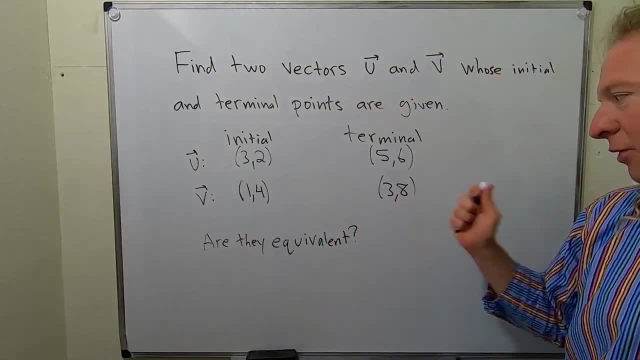 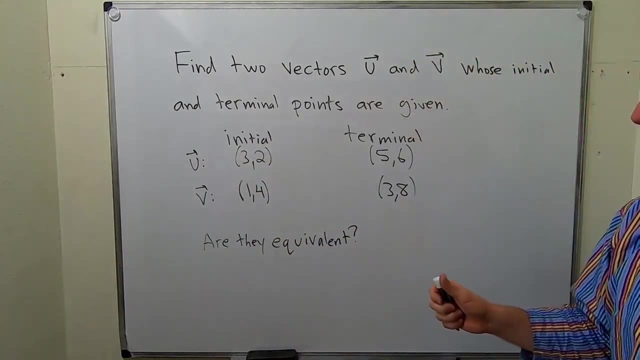 And the vector v, with initial point 1, 4 and terminal point 3, 8. And we have to find the vectors and determine if they're equivalent. So to find the vectors, all we do is we subtract. It's always terminal minus initial. 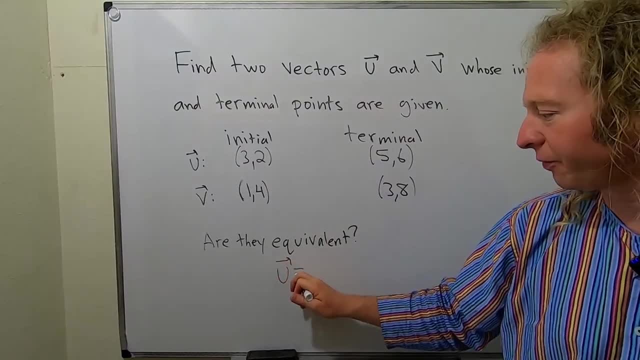 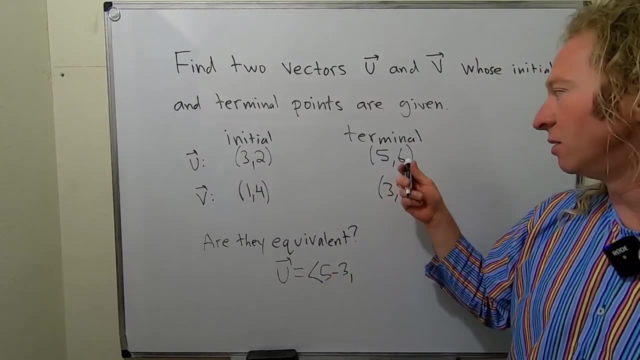 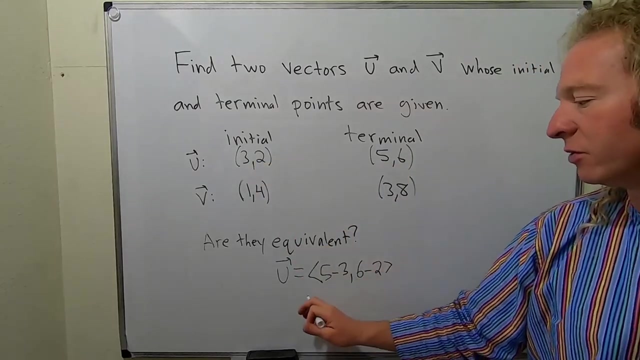 Terminal minus initial. So for u it would be 5 minus 3.. So 5 minus 3.. And then you subtract the second coordinate or the y component, So 6 minus 2.. So 6 minus 2.. So this is equal to. 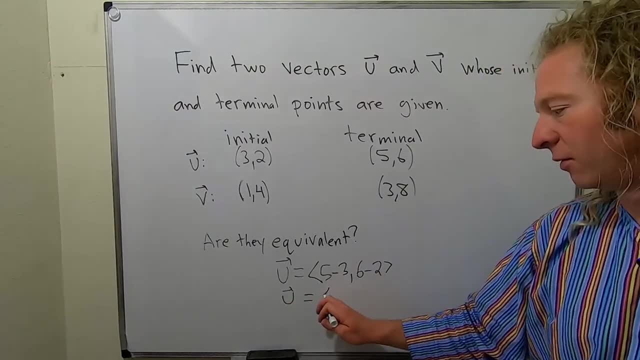 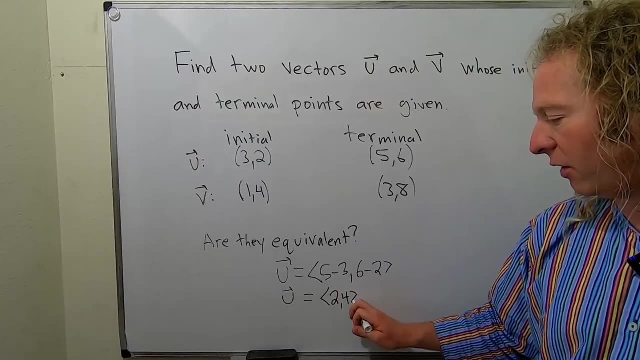 Let's see, Let's see, Let's see: 5 minus 3 would be 2.. So angle bracket: 2.. And 6 minus 2 would be 4.. So 4.. And there is our u. So that is our first vector u. 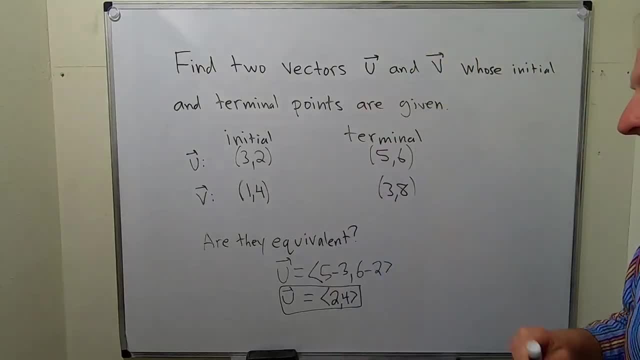 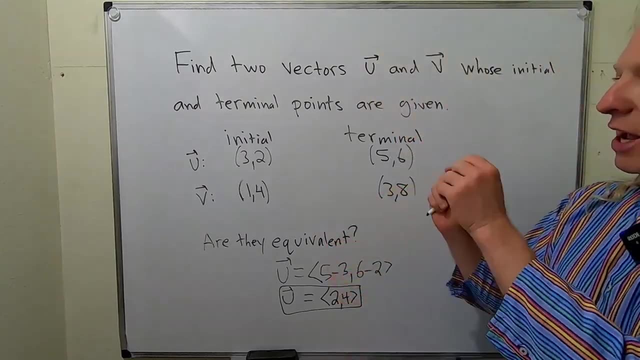 It's really, really important, the whole terminal minus initial thing. You might think, oh, it's really simple. It's important for understanding later, Like if you want to understand certain derivations in calculus 3, it's really important to have this notion of terminal minus initial down. 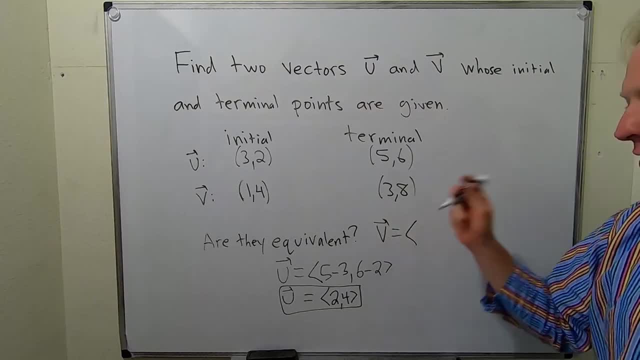 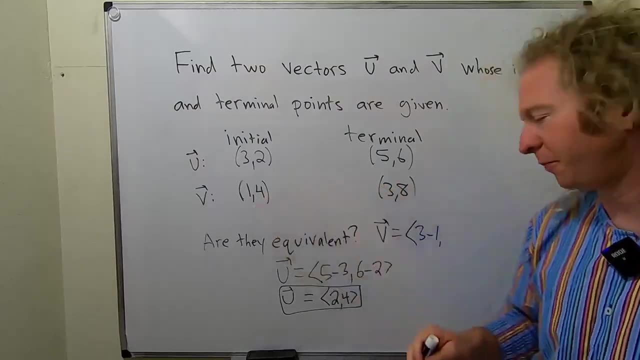 So v. So it'll be terminal minus initial. So 3 minus 1.. So 3 minus 1. And you can skip steps. I'm just showing extra steps And 8 minus 4.. So 8 minus 4.. 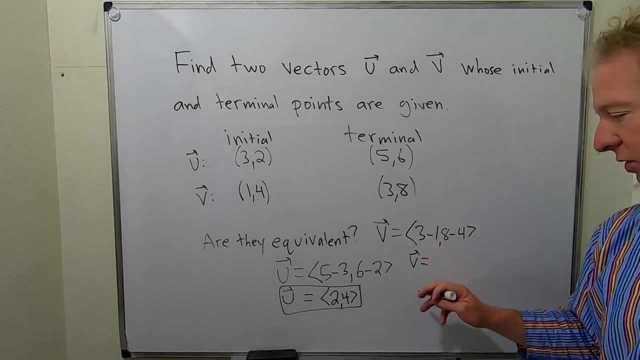 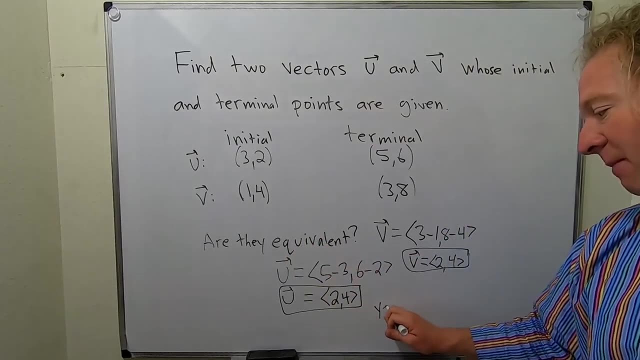 Beautiful stuff. So v is going to be equal to 3 minus 1 is 2. And 8 minus 4 is 4.. Oh look, They're the same. So the answer is yes, they are equivalent. You might be wondering: what does that mean? 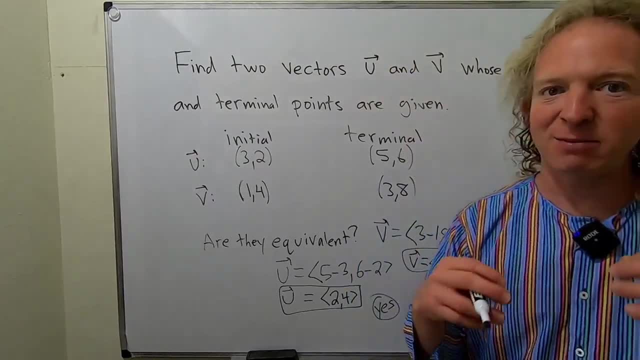 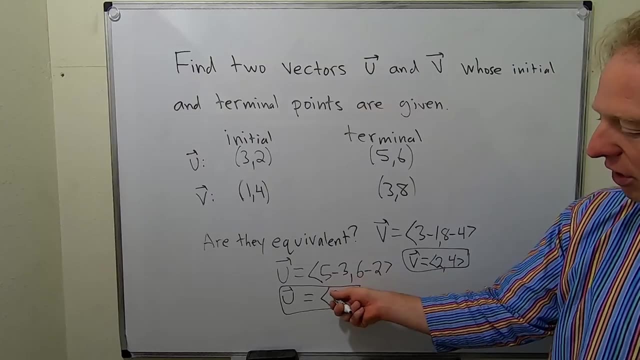 What does it mean to be equivalent? So two vectors are equivalent if they have the same direction and length. In other words, when you write them like this, they're going to be exactly the same. So this is a vector whose initial point now. 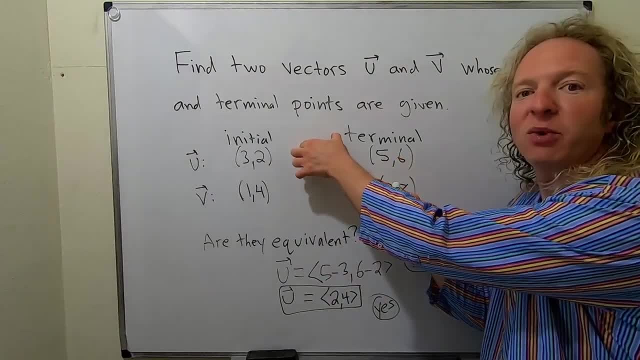 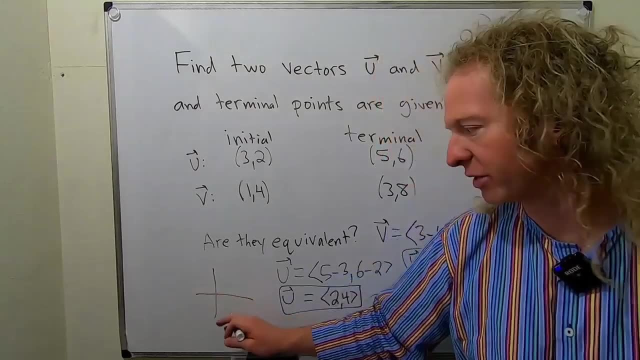 is at the origin. So we took this vector in the plane and we've kind of shifted it down to a vector whose initial point is at the origin. So if you were to sketch this vector, it would look like this: 1, 2, 1, 2,, 3, 4.. 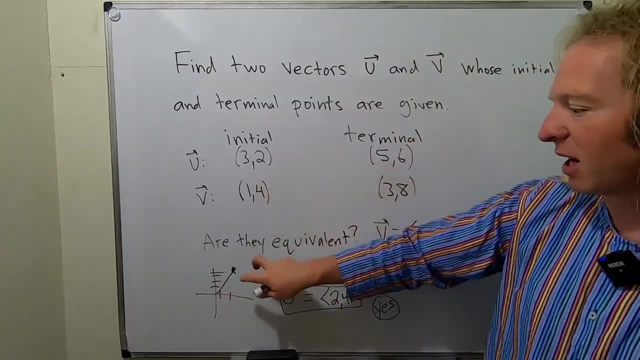 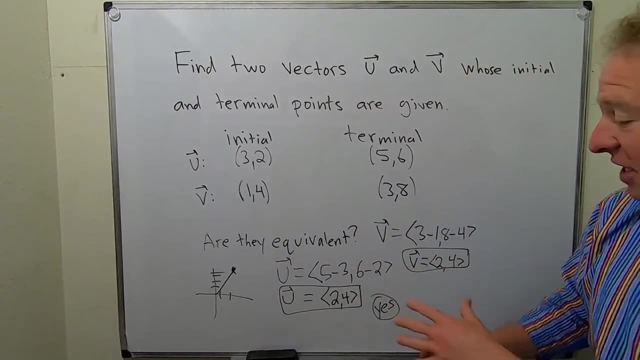 And so that would be the vector. So these vectors here are the same, except they're in different places on the plane, But they all have the same length and direction. Therefore they're equivalent. So if you get a different answer here, the answer would be no. 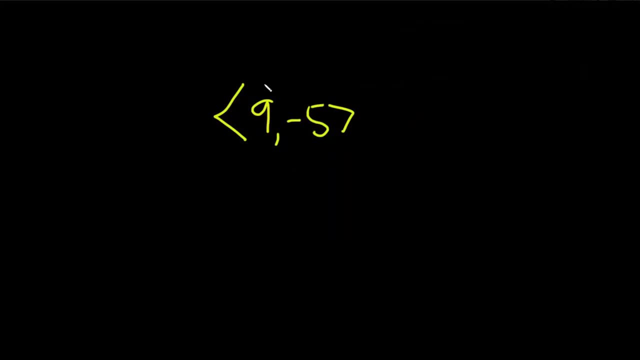 So Hope this video has been helpful. Find a unit vector that has the same direction as this one. So to find a unit vector in the direction of this one, all we have to do is take this vector here and divide it by its magnitude. 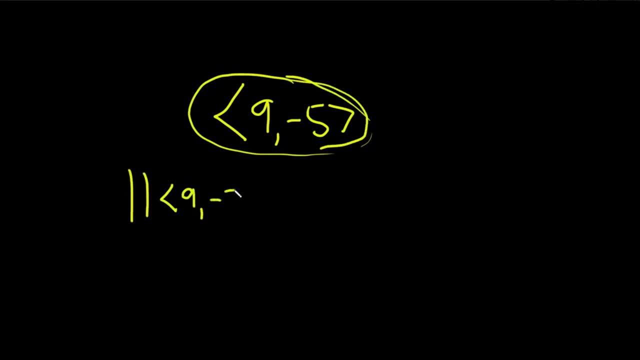 So we'll start by finding the magnitude of this vector. So to do that, the formula is that it's the square root of, And then you just take each component and you square it, So it's 9 squared plus negative 5 squared. 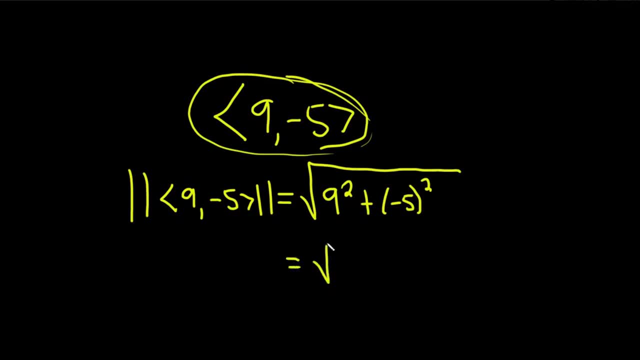 Just square each of the components. So 9 squared is 81.. And negative 5 squared is 25.. If you add these numbers you get 106.. So this is the length or the magnitude of this vector. So to find a unit vector that has the same direction as this one, 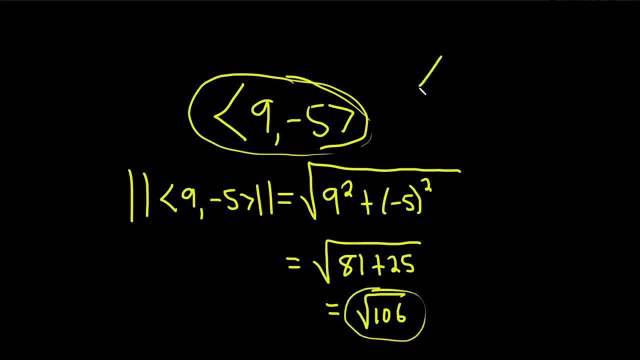 we just take this vector and we divide it by this. So basically you just divide each component, So it would be 9.. And then this is our unit vector. So this would be 1 over the square root of 106, comma negative, 5 over the square root of 106.. 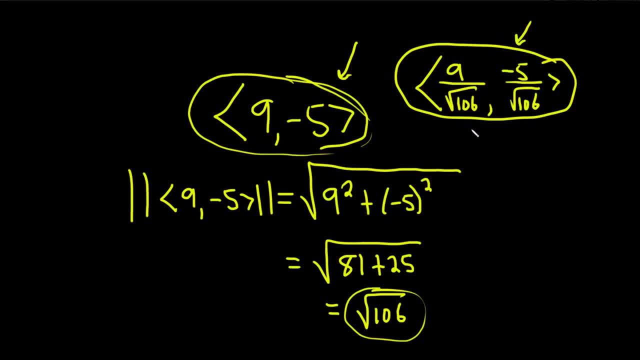 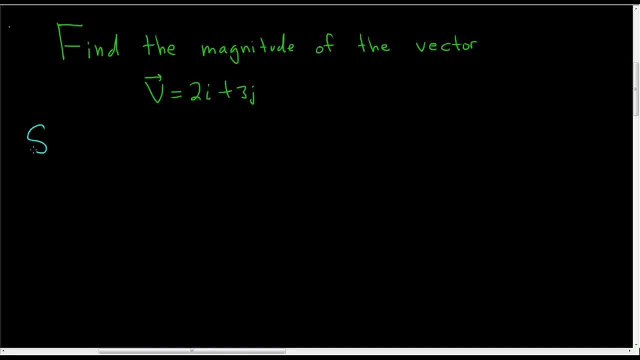 And this would be a vector that has the same direction as this one, but this is a unit vector. That means that the length of this vector is equal to 1.. I hope this video has been helpful. Find the magnitude of the vector v equals 2i plus 3j. solution. 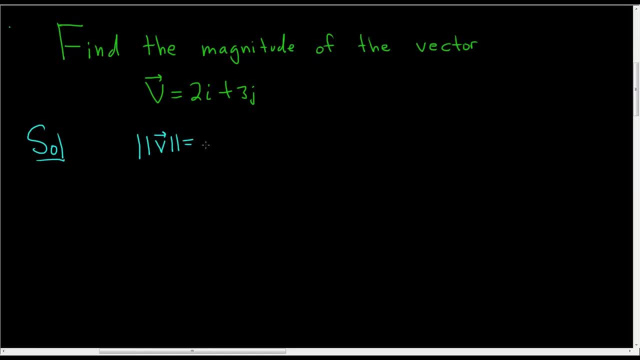 So the formula for the magnitude of a vector is the square root of a squared plus b squared, where V is equal to the vector whose first component is a and its second component is B. so in this problem we can write this vector in component form, so 2 comma 3, and then just use the. 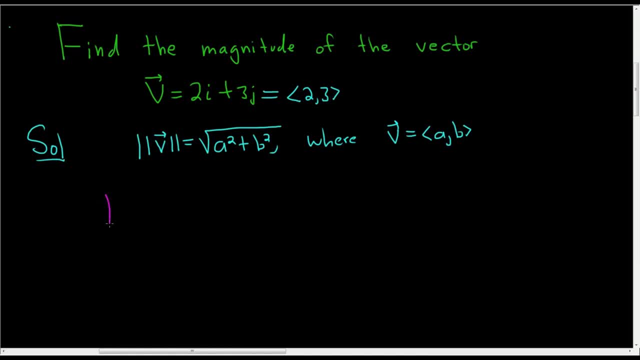 formula. so let's go ahead and do it. so the magnitude of V is the square root and in this case a is 2 and B is 3, so 2 squared plus 3 squared, super easy. so 2 squared is 4 and 3 squared is 9, so we end up with the square root of 13 and 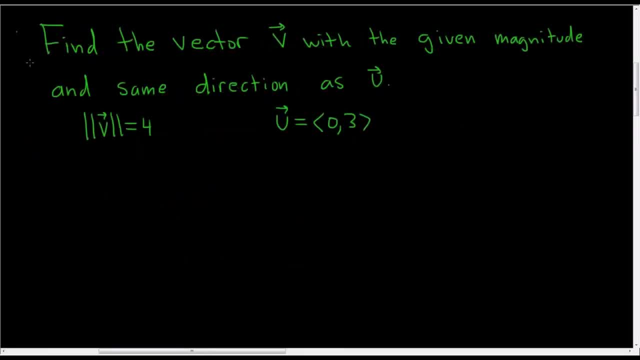 that's it. we're being asked to find the vector V with the given magnitude. so here the magnitude is given to be 4, so this is the magnitude and same direction as this vector here. so let's work it out. so first we will find a unit vector in the same direction as you, so we will first. 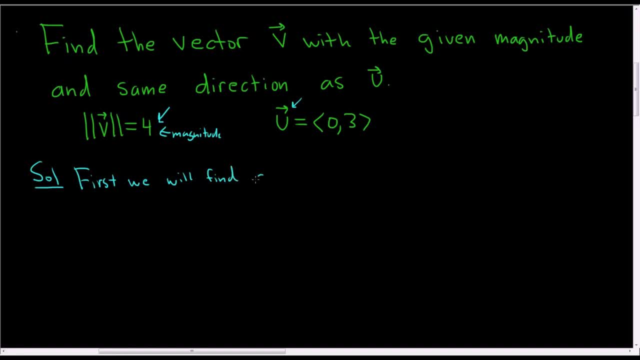 we will find a unit vector in the same direction as you. that'll be the first step. so step 1: we'll find a unit vector in the same direction as this one, and step 2 will multiply our result. so multiply our result, our new vector, by 4, and then we'll be done. 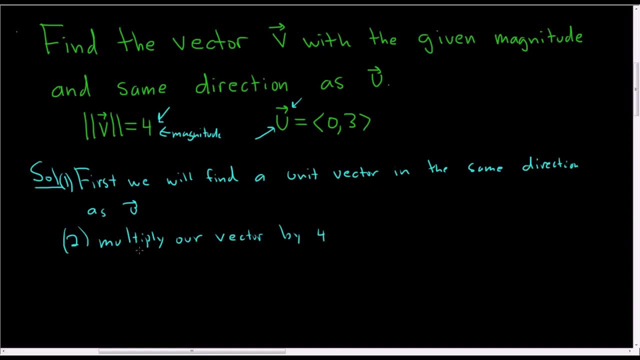 right, because then we'll have a vector in the same direction as you with magnitude 4. so first let's find the unit vector in the same direction as you. so the formula for that is you divided by the magnitude of you. this will be a unit vector in the 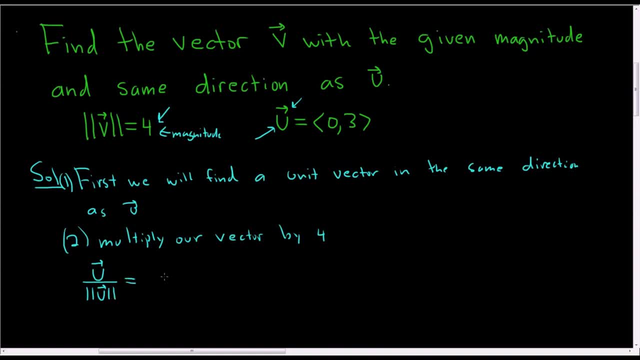 same direction as you. so you can write this as 1 over the magnitude of you and you can write this as the square root of times you. so this is 1 over now the magnitude of U is the square root of, and you just square this, so 0 squared you. 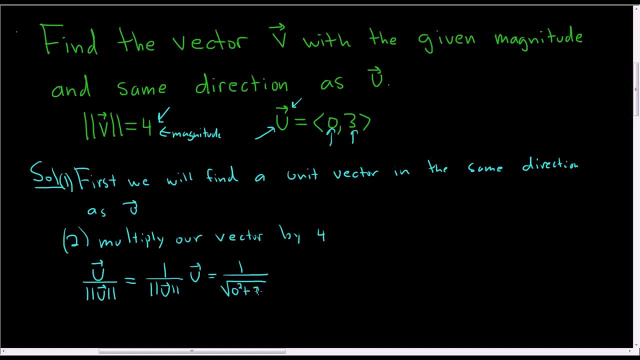 add, and then you square the 3. so 3 squared, 3 squared, that's a 3, and then U is 0- 3, so this is 1 over the square root of 9, and then we still have 0, 3, and then 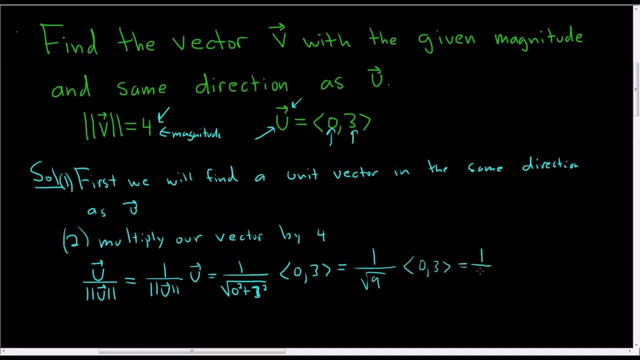 So this is 1 over 3.. We still have 0, 3.. And finally, just distribute: 1 third times 0 is 0, and then 1 third times 3 is 1.. So there is our unit vector in the same direction as u. So that was step 1.. Step 2, we'll just multiply this by 4 and we'll be done. 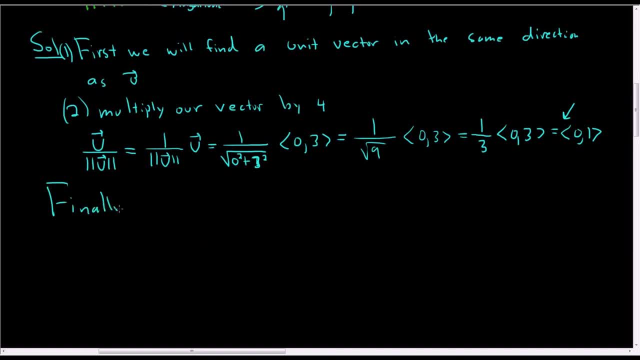 So finally make it seem like a long problem- is 4 and then times our vector. So this will be: 4 times 0 is 0 and then 4 times 1 is 4.. So that is the final answer. I hope this helps. We're given two vectors and we're asked to find the angle between them. 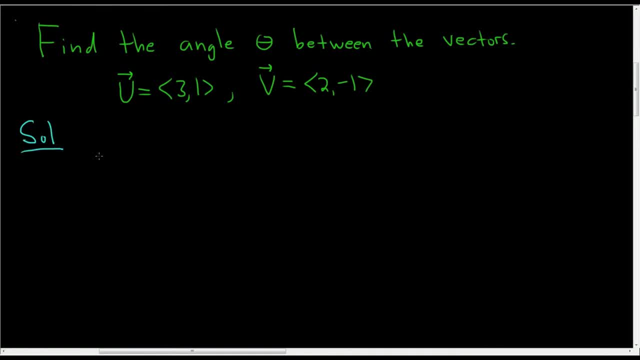 Let's go ahead and do it. So there's a formula. It basically says that the cosine of the angle between the vectors, which is called theta, is equal to the dot product of u with v divided by the magnitude of u, and that's being multiplied by the magnitude of v. 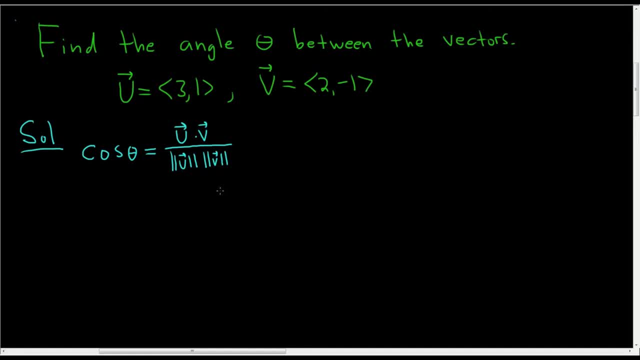 So we can do this all at once or we can do it one step at a time. Let's do it one step at a time. So if we look at u dot v well, to compute the dot product, we need to do this one step at a time. So if we look at u dot v well, to compute the dot product, 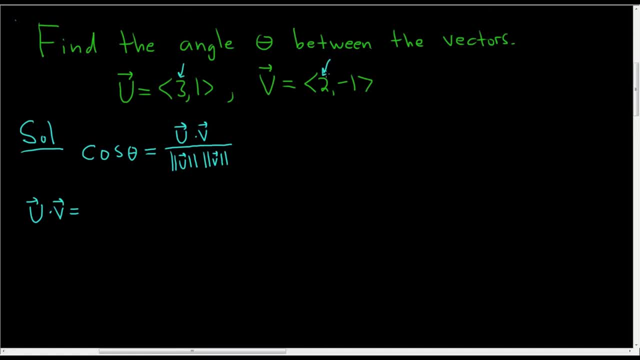 we need to do this one step at a time. So if we look at u dot v, well, to compute the dot product we multiply the corresponding coordinates, So we multiply the first components, so 3 times 2, and then we multiply the second components, so 1 times negative 1, so plus 1 times negative 1.. 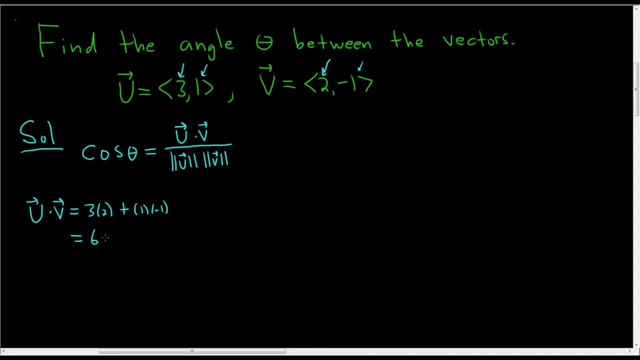 This ends up being 3 times 2 is 6 and 1 times negative. 1 is negative 1, so we get 5.. So the dot product of u with v is equal to 5.. Let's go ahead and find the magnitude of u. 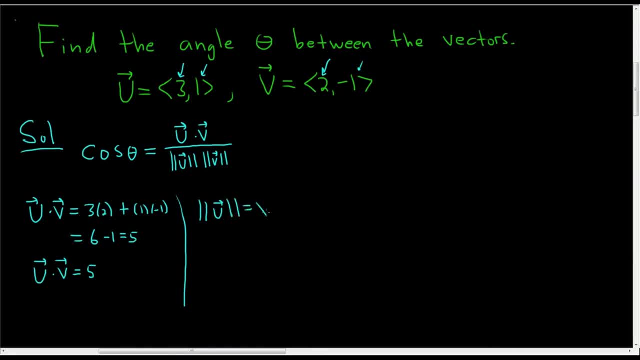 So the magnitude of u, that's equal to the square root. And you just square the components and add, So 3 squared plus, and then 1 squared, So you end up with 9 plus 1, which is equal to 10, so the square root of 10.. 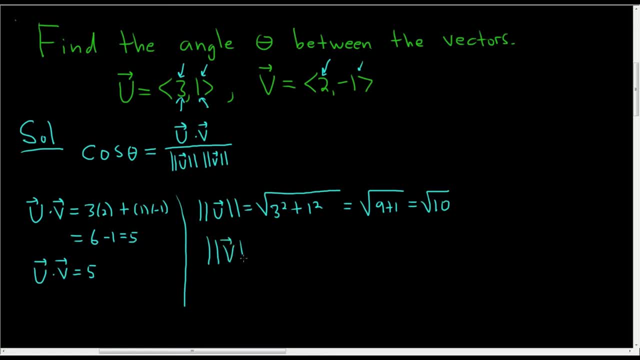 To find the magnitude of v. it's the same thing. You square the components and add, So it's the square root of two squared, So two squared plus. and then the second component is negative one, so negative one squared, So we end up with four plus one, which is equal to the. 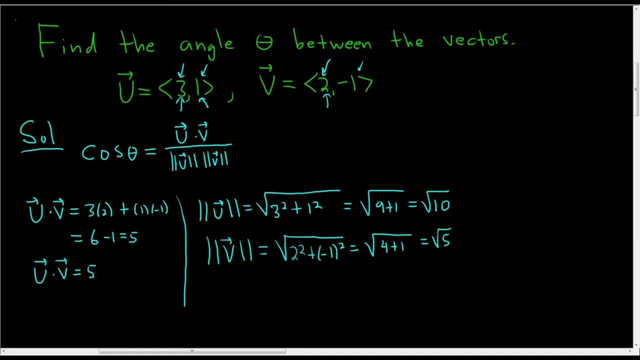 square root of five. I think now we're in a good place to go back to the formula. So this is equal to, let's see, u dot v. we said that was five, So five the magnitude of u. well, that's the square. 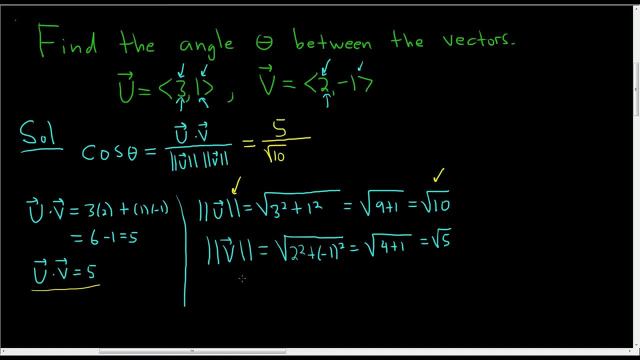 root of 10.. And the magnitude of v? well, that's the square root of five. So this is equal to five over the square root of 50.. This is equal to five, To simplify the square root of 50.. The way I do, 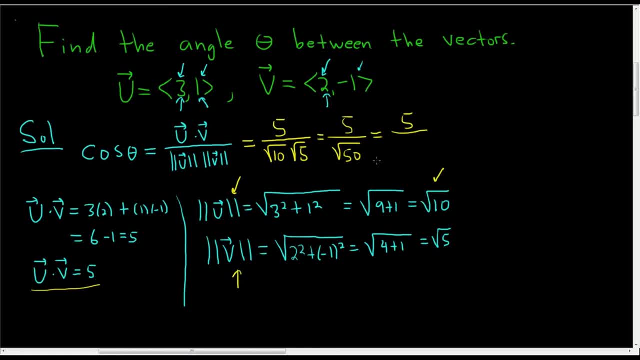 it is. I asked myself: what is the largest factor of 50?? That's a perfect square. Well, 25.. So this is square root of two times the square root of 25.. So this is five over the square root of two times five. fives cancel, So we get one over the square. 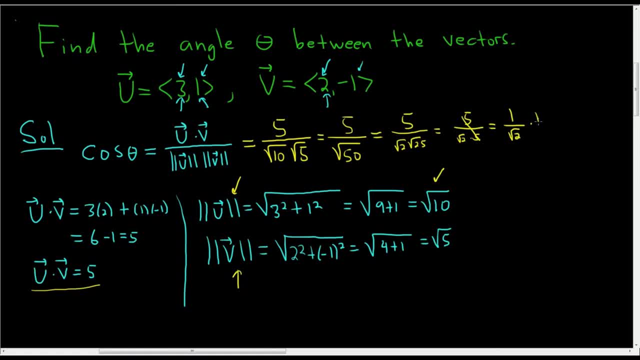 root of two. This can be rationalized: you multiply by the square root of two over the square root of two, And so we get the square root of two over two. So we have that the cosine of theta is equal to the square root of two over two, And that means that theta is equal to pi over four. that's the. 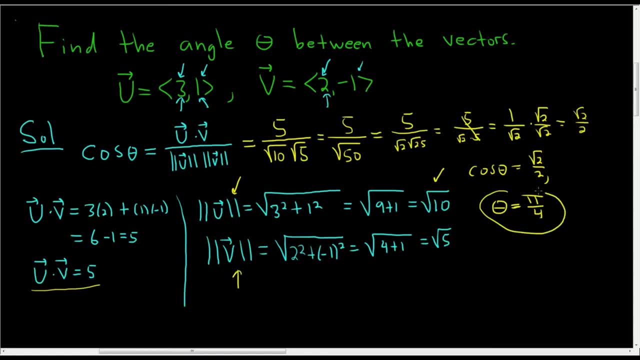 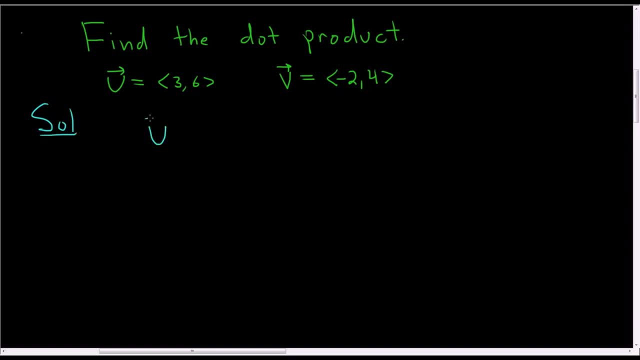 angle we want, That's between these vectors. I hope this helps. We're being asked to find the dot product. This is extremely easy. So we have the vector u and we're finding the dot product of that vector with the vector v. So this is equal to the vector u, which is three comma six, And we're taking the dot product. 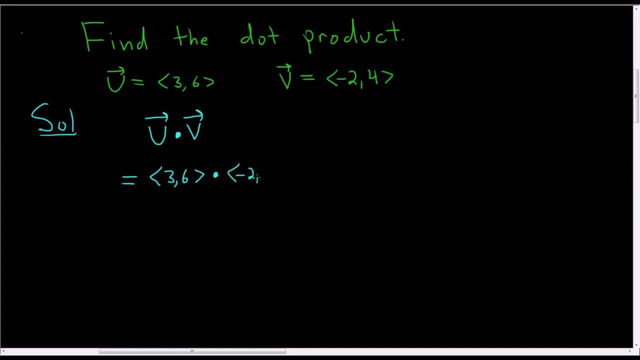 of that with the vector v, which is negative two comma four. And so to find the dot product, you just multiply the first components, so three times negative two, And then you add, and then you multiply the second components, So six times four. So again, you just multiply three times negative two, so the first. 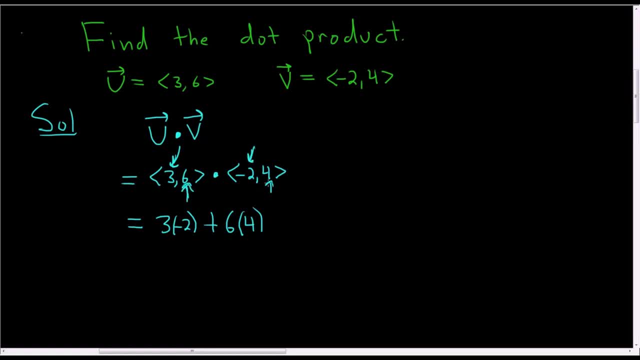 components, and then you multiply these second components. So six times four, three times negative two is negative six, And six times four is 24.. So negative six plus 24.. That's going to be equal to 18.. And that's how you find the dot product of two vectors. That's it. 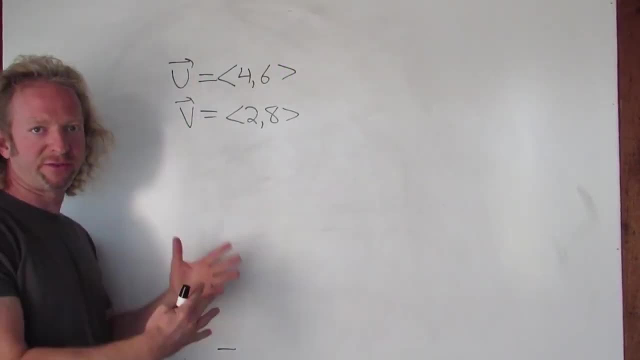 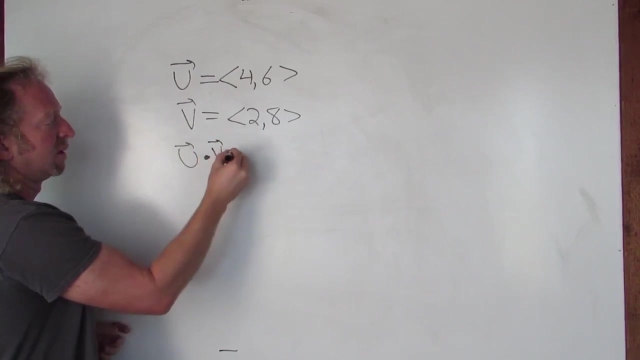 Hey everyone. So in this video we're going to find what's called the dot product of these vectors. So to find the dot product, you write u and you put a dot and then v. All you have to do is multiply the x's. 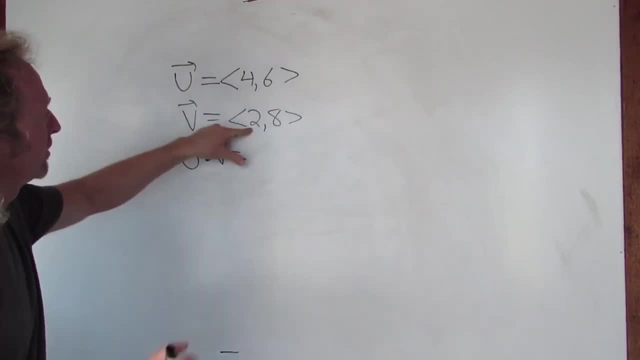 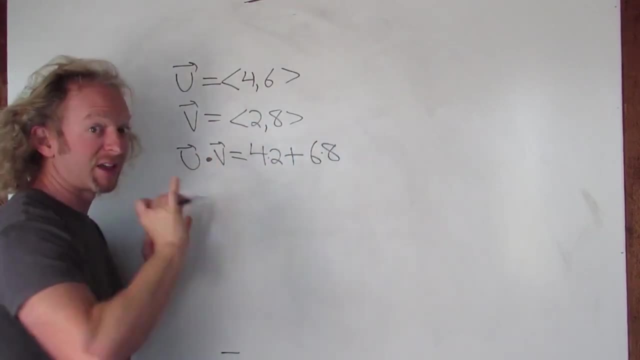 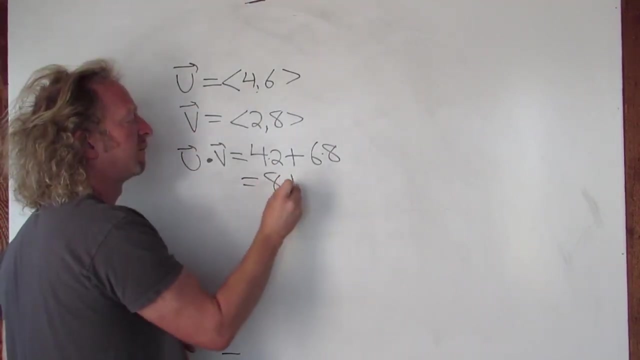 and add, and then multiply the y's and add. So you do four times two and you put a plus sign. Then you do six times eight. That's it. Subtitles by the Amaraorg community. So it's just four times two plus six times eight. Four times two plus six times eight. Four times two is eight. Six times eight is 48.. So that gives you 56.. 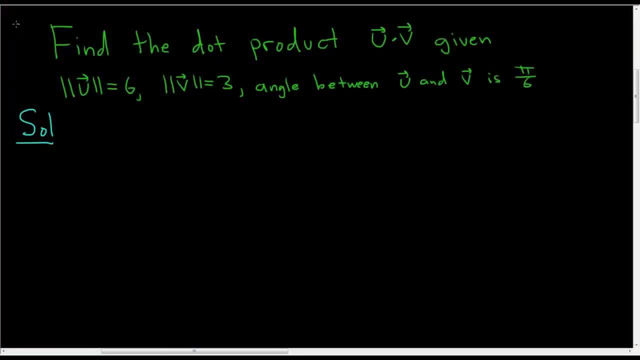 And that's it. That's how you find the dot product, Being asked to find the dot product. except we're not given the actual vectors. Instead we're given the magnitude of the vectors and the angle between them. So there's a formula It says: if you have cosine theta, this is equal to the dot product of